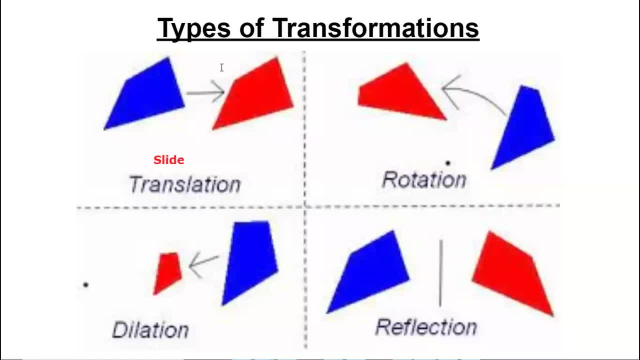 is a slide, And then we have the rotation, which is a turn, And we have the reflection, which is a flip And dilation, And then we have transformations which I mentioned you're going to be learning about in another module. 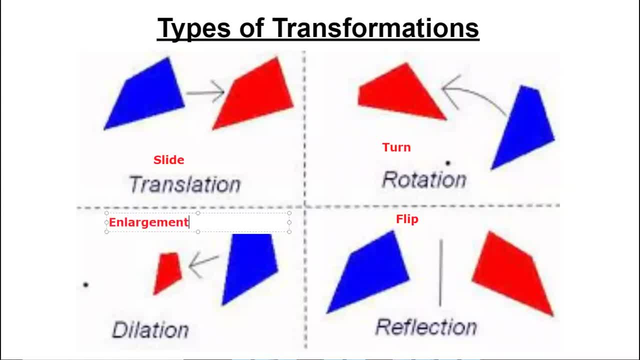 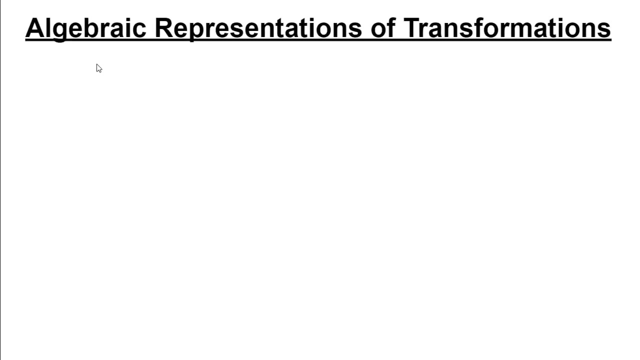 That is an enlargement or a shrinking. I spelled shrinking wrong. There we go. So those are the four types of transformations. So let's talk about how we would represent these transformations algebraically. You've learned some of the rules for how the x and y coordinates change when doing rotations. We talked about that in the lesson before this one. It's good idea to go back and review that. 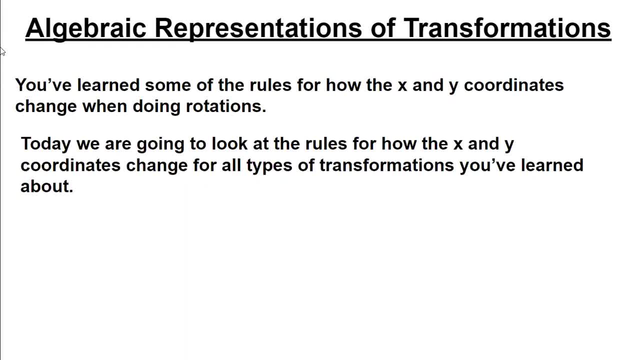 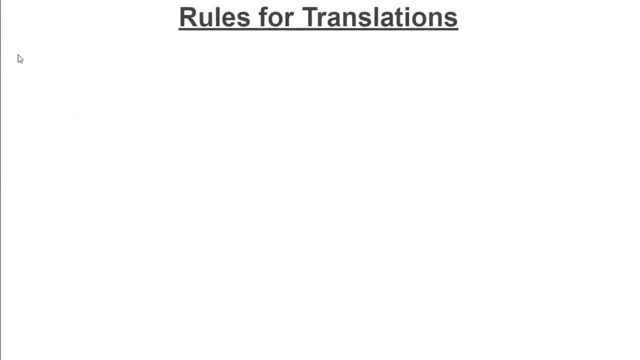 Today we're going to look at the rules for how the x and y coordinates changed for all types of transformations that you've learned about. So we're going to talk about rules for translations. So this is a translating. Again, it's a slide, And later, when you get into high school, you're going to be talking about vectors and what that all means. 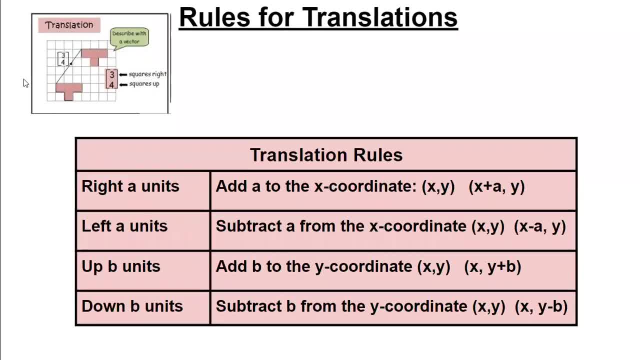 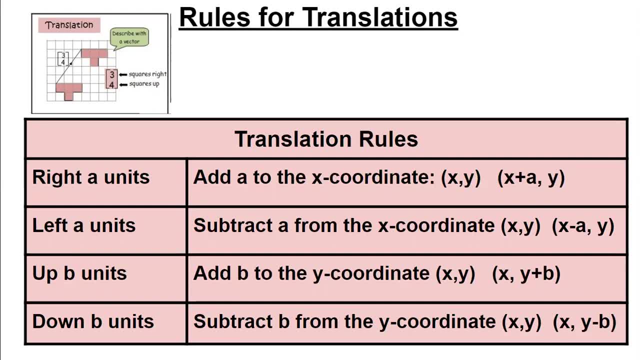 So that'll be interesting. So here's the translation rules. So if the translation figure goes to the right, a certain number of units in here we're calling it a units, a units, Then we're going to add a to the x coordinate, And that makes sense, right? 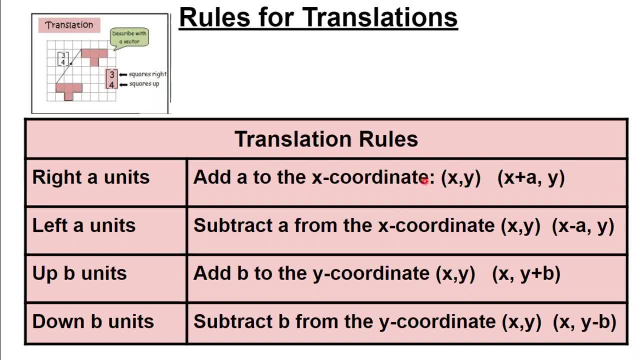 If it's going to the right, the x number is going to get bigger by the number of units it moves to the right. So we say that in modeling terms, x plus a and then y will stay the same. If we go left a units, a certain number of units, then we're going to subtract the a from the x coordinate. 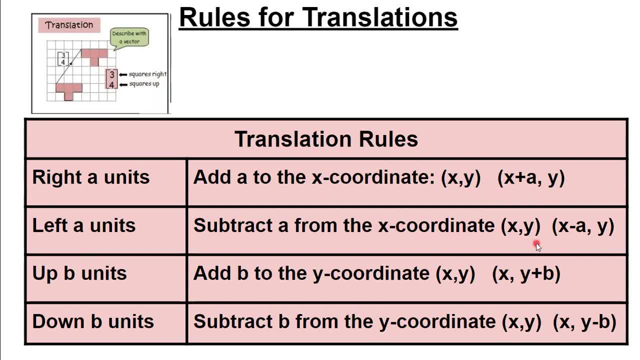 That makes sense. Our x value should get smaller. So from x to y it changes to x minus Y minus a and y stays the same. If we go up b units, we're going to add b to the y coordinate. That makes sense. As you go up, the y value should increase. 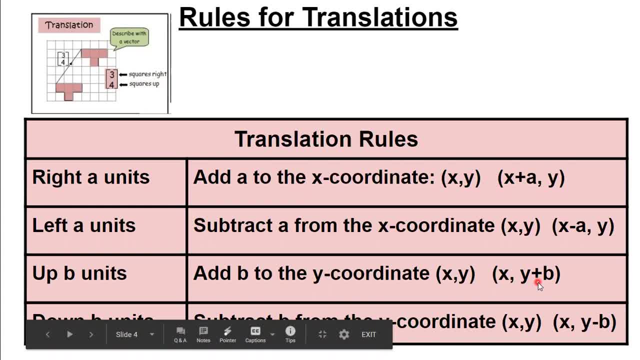 X stays the same and we add b to y, So y plus b. And finally, if we go down b units, we're going to subtract b from the y coordinate, which makes sense. The y value should get smaller if you're moving down. 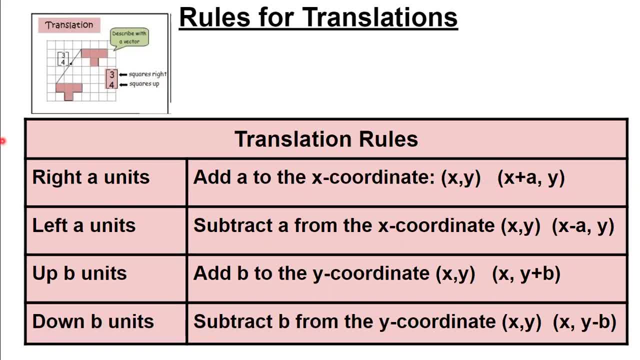 So it'll be x comma y, Y minus b. Those make sense. They should make sense to you, as far as visually, if you think about them in your head. Okay, so let's see how this would work. So here's our translation rules. 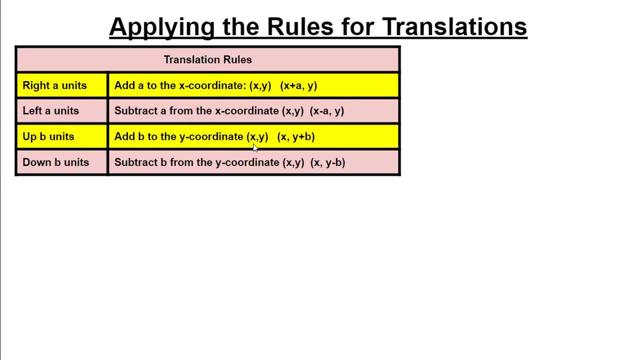 Again. I've put them up here. They were the ones on the previous screen And we have triangle x, y, z. It has vertices of x at 0, 0,, y at 2, 3, and z at 4, negative 1.. 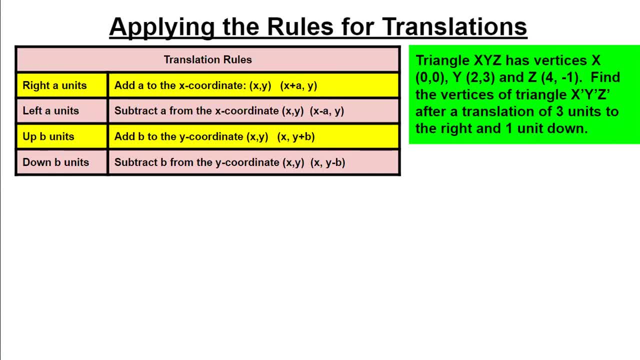 Find the vertices of triangle x prime, y prime, z prime, after a translation of three units to the right and one unit down. So I've highlighted in yellow the two rules we're going to be using. It's going to the right three units. 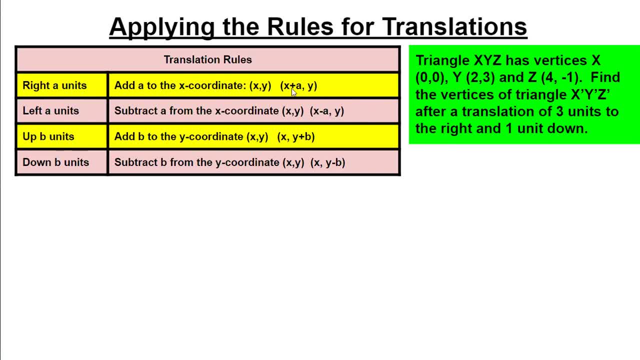 So that's a unit. So we're going to be adding three to x And it's going down to the right and one unit down. Hold on just a sec. I highlighted the wrong one. Okay, I fixed it. I highlighted the one above it. 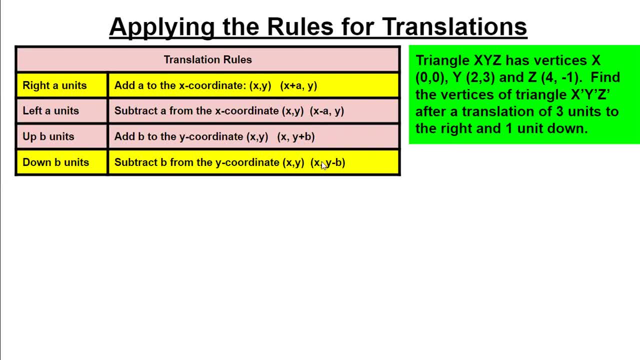 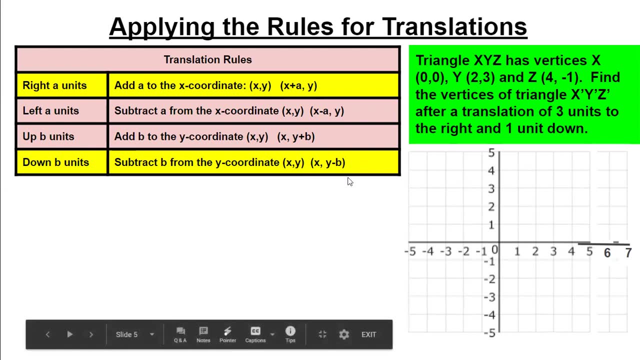 So it should be down b units. So that means we're going to subtract one unit from y. Okay, so here is our coordinate plane And ignore this little thing here. It's as best I could get the line to line up. I had to have a couple extra numbers there to do our problem. 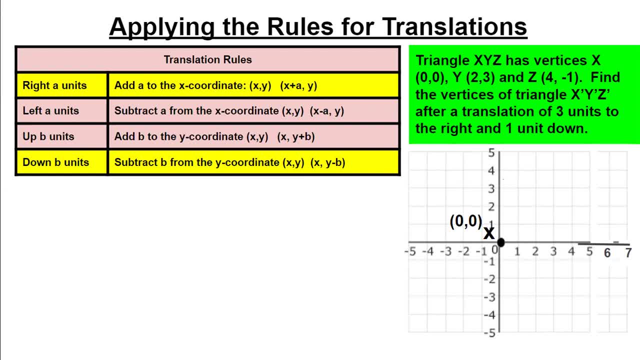 Okay, so we're going to plot: x is at 0, 0.. Y is at 0, 0.. Y is at 2,, 3. And z is at 4, negative 1.. Connect the dots And there is our triangle: x, y, z. 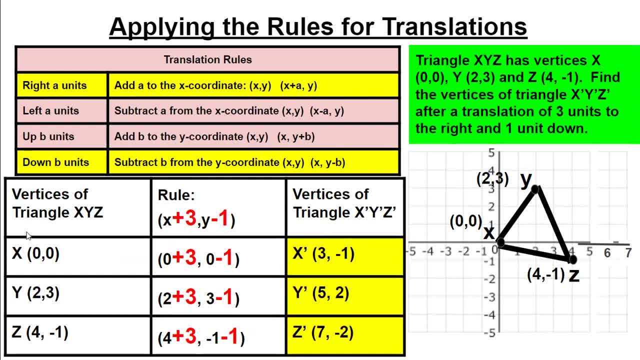 Now we're going to apply the rules. Here's what the vertices were. Let me grab my spotlight. They were right here. These were the vertices. And now here's our rule. We're going to be going to the right three, So we're going to add three to x. 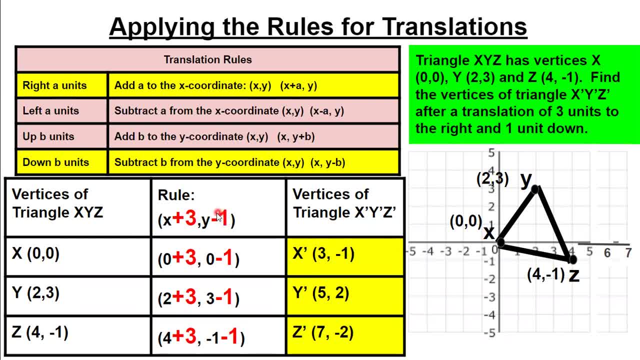 We're going to be going down. So we're going to subtract one from every y value. So we had zero, We're adding three. We had zero, We're subtracting one. That results in zero plus three is three. Zero minus one is negative one. 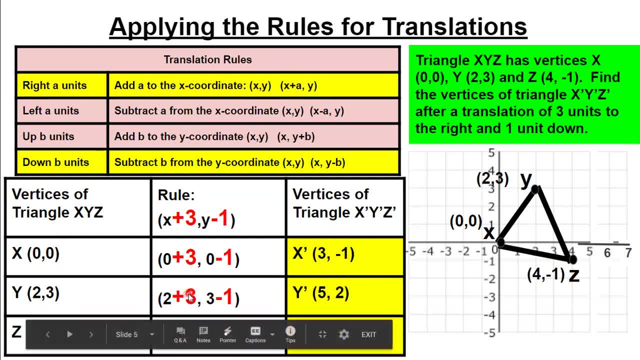 On the y values, we have two. to begin with We added three. We had three. for the y value We subtracted one. So two plus three is five And three minus one is two. For z, we had four, And then we add three to that. 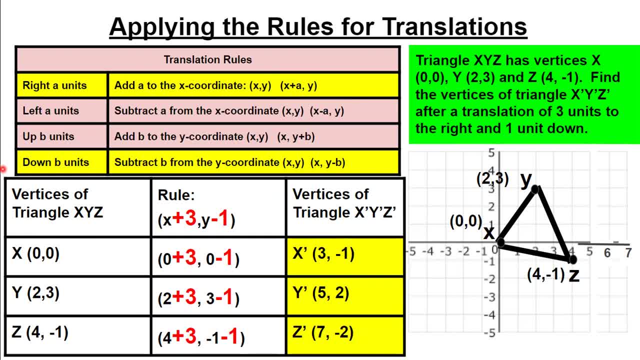 And then we had negative one And, be careful, we subtract one So that results in: four plus three is seven, And negative one minus one is the same as negative one plus negative one, which is negative two. So let's plot our new x prime, y prime, z prime points. 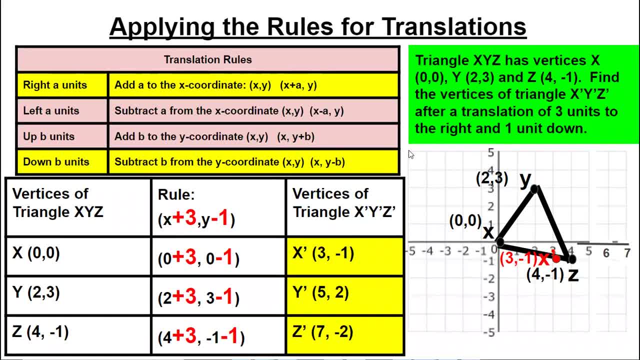 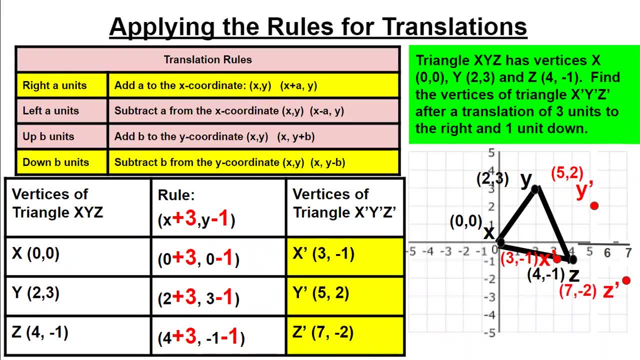 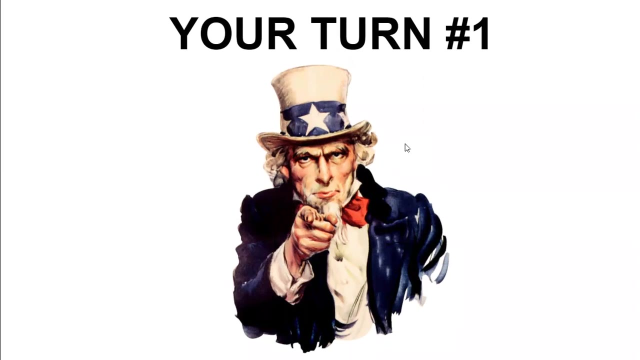 There we have x- prime three, negative one, Y- prime five, comma two, And z- prime seven, comma, negative two, And then we connect the dots And that is a translation of three units to the right and one unit down. Okay, you get to try some translations, finding the coordinate values. 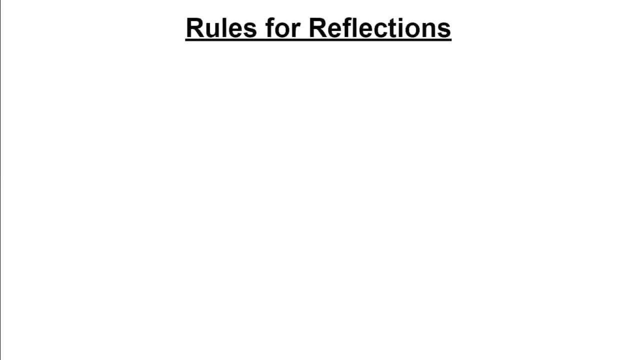 Okay, welcome back. Let's continue with rules for reflections. Okay, that's a reflection. A reflection is a flip, So notice how you can have a flip. This is this picture. for a minute You can have a flip across the x-axis or across the y-axis, or across the y equals x. 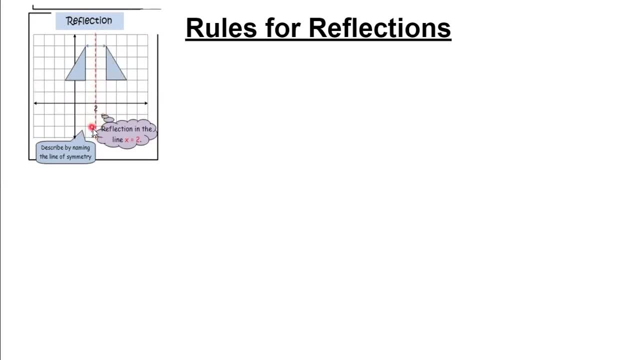 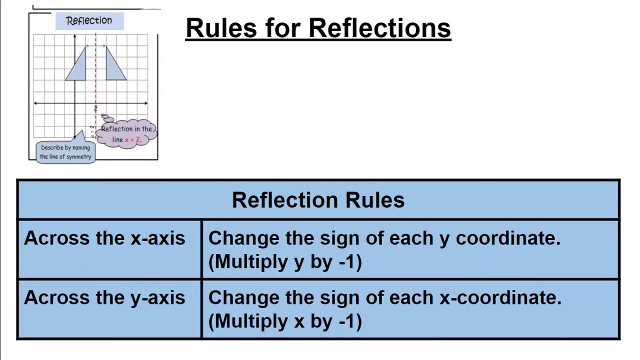 In this case it's a flip across. x equals two, So that's interesting. You can have any line anywhere and do, Okay, reflection across that line. Here are the rules for reflection. If you go across the x-axis, you're going to change the sign of each y-coordinate. 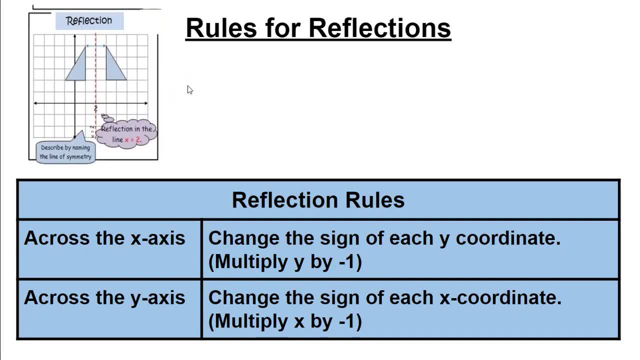 To change the sign you multiply by negative one Across the y-axis. you're going to change the sign of the x-coordinate and you're going to multiply the x by negative one. So just be aware it's the opposite of what you think. 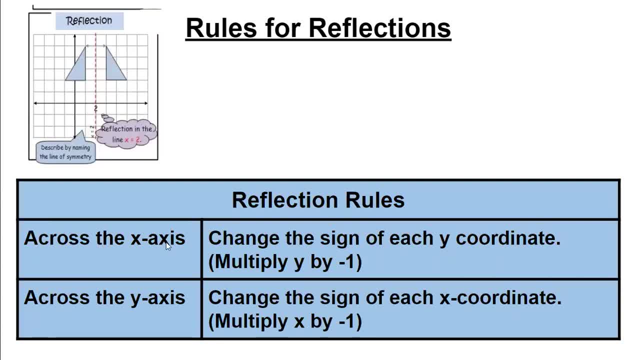 So as you go across the x-axis, when you flip your shape, you're going to change the y-coordinate sign. When you go across the y-axis and flip your shape, you're going to change the x-coordinate sign. So just the opposite. 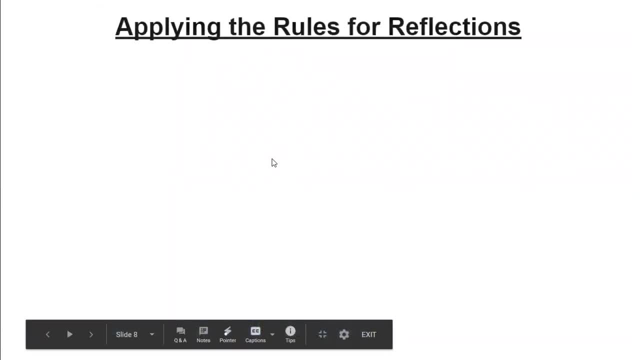 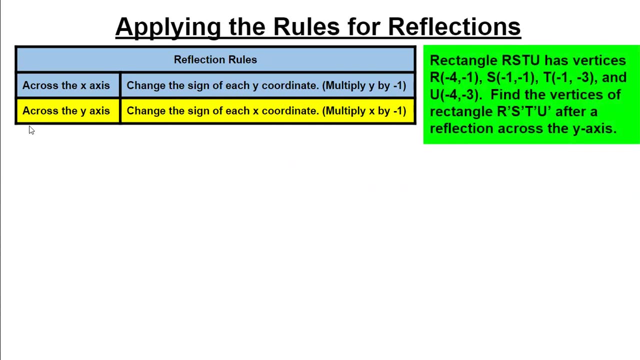 So let's see this in action. So here's our rules in smaller format. Here's our problem: Rectangle rstx. RSTU has vertices: R negative 4, negative 1, S negative 1, negative 1, T negative 1, negative 3, and U negative 4, negative 3.. 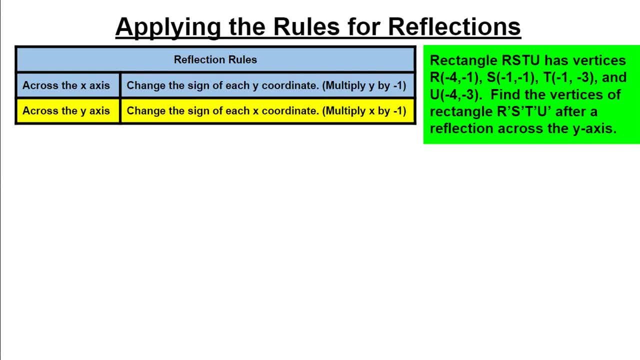 Find the vertices of rectangle RSTU after a reflection across the y-axis. There's our graph, So we're plotting the points- There's R, there's S, there is T and there is U- And we connect the dots and there is our rectangle. 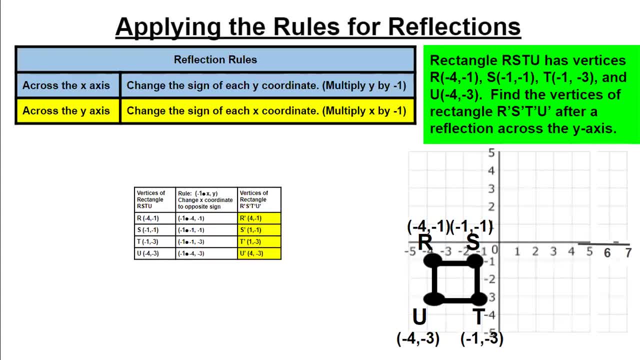 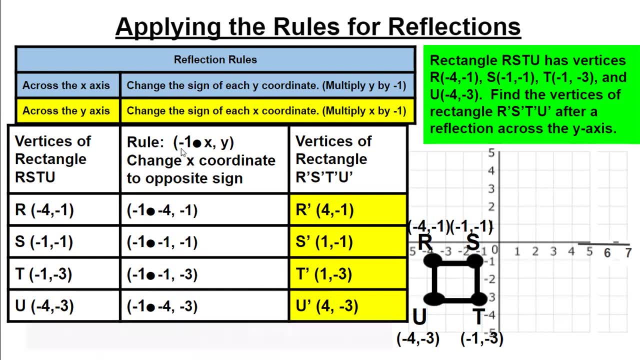 It's more like a square, but it's supposed to be a rectangle. So here are the vertices of the original rectangle: RSTU. What's the rule? The rule is we're changing to the opposite sign for X, right, Because we are flipping it across the y-axis. 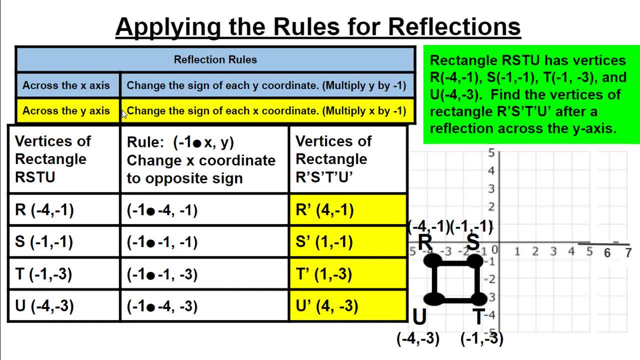 So the highlighted yellow box is our rule for this problem, So I'm showing it here. It's negative 1 times the X, Because if you multiply negative 1 times any number, it will change. If X is negative, it will change it to positive. 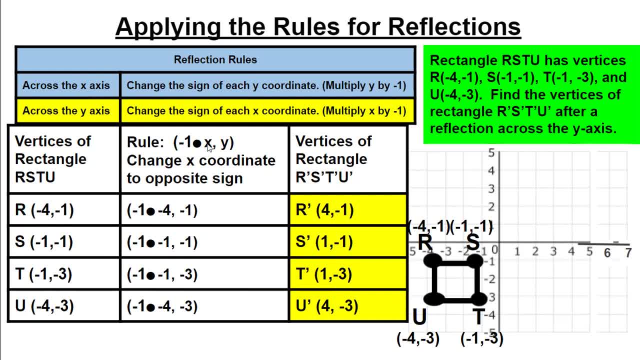 If X is positive, it will change X to negative. So basically you're changing to the opposite sign. So if R is negative 4, it's going to become positive 4.. Y will stay what it was. If S is negative 1, it's going to become positive 1.. 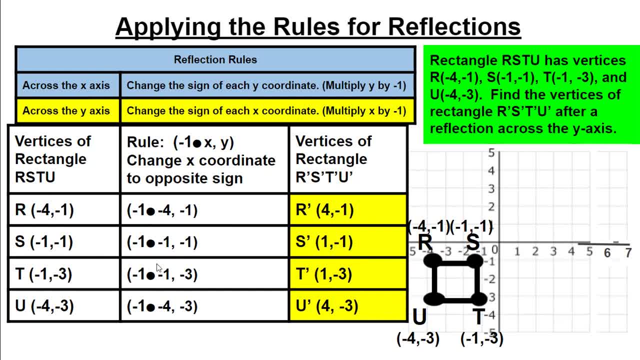 And the Y will stay what it was: Negative 1 for T, for the X is going to become positive 1. Y stays the same And for U, negative 4 is going to become positive 4, and negative 3 stays the same. 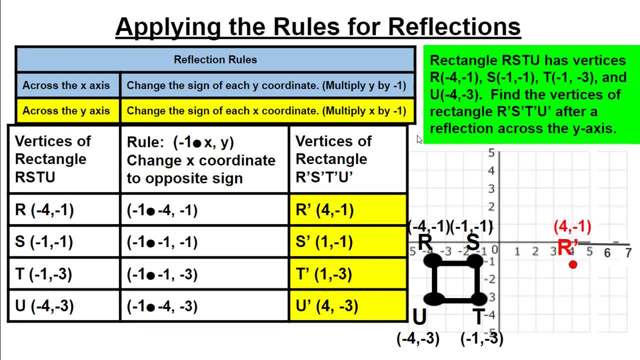 Then we plot our new vertices: 4, negative 1.. S is at 1, negative 1.. T is at 1, negative 3.. And U is at 4, negative 3.. And then we plot it and you can see that that is a flip across. 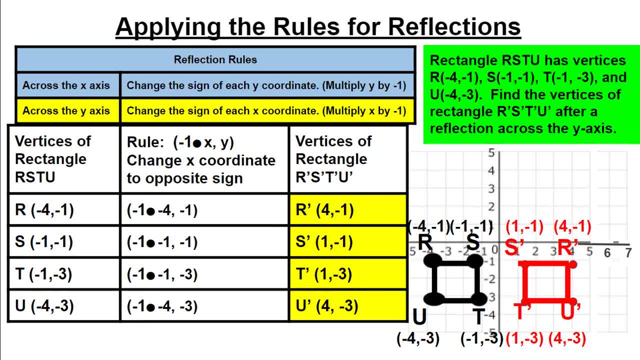 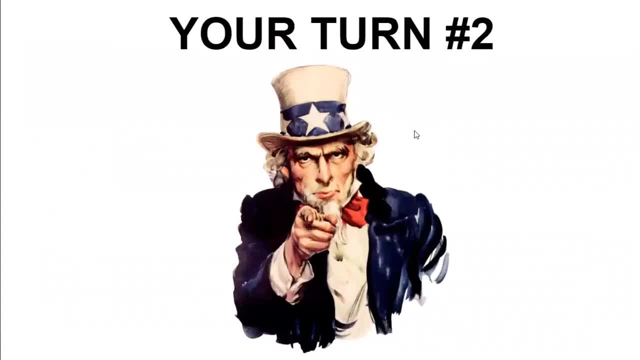 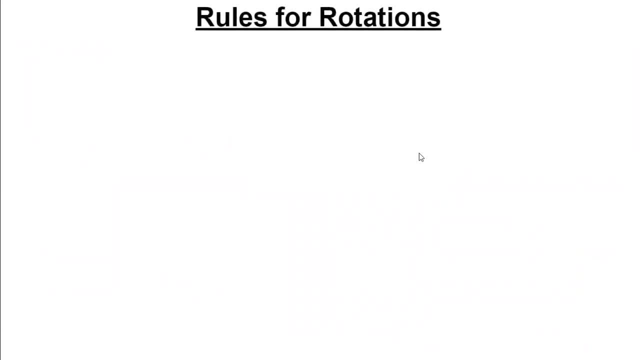 The 1. Y axis And it is reflected. Okay, you get to try some reflections. I'll see you back in a moment. Okay, welcome back. We're going to do some rules for rotations, So here's a rotation. 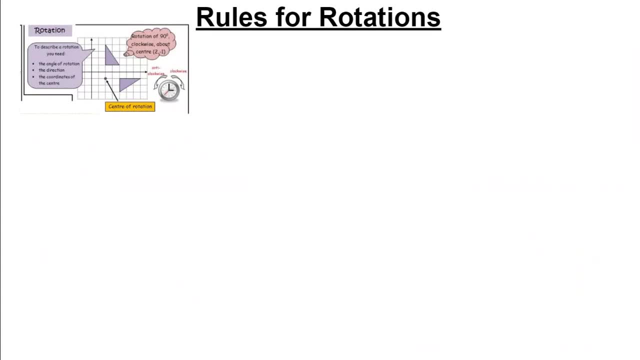 A rotation is a turn, And notice how you have to know certain things for a rotation. You have to know the angle of rotation Like: is it 90 degrees, Is it 180 degrees, Is it 270 degrees? You have to know the direction, clockwise or counterclockwise. 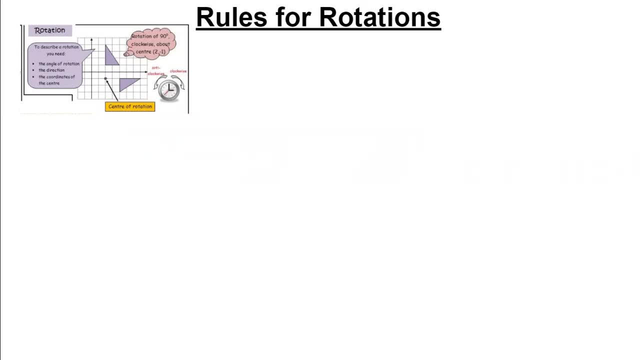 You have to know the coordinates of the center. We've been flipping or we've been rotating everything around the origin 0, 0. When you get into higher level geometry you will be rotating around other points besides 0, 0. 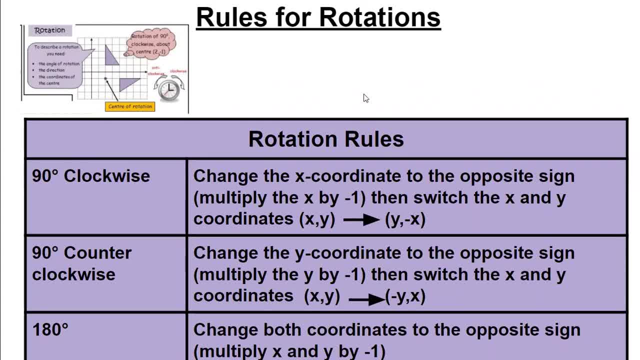 Okay, here are our rotation rules. These are the ones from our previous video, So if you have a 90 degrees clockwise rotation or a 270 degrees counterclockwise rotation, remember they're the same thing. So I can add that in here. 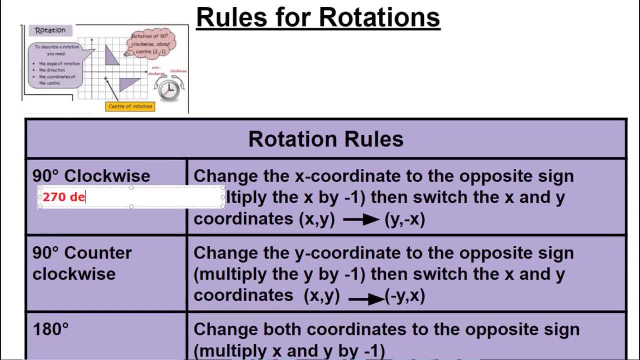 I'll put that in here, just to have it: 270 degrees counterclockwise is the same as a 90 degrees clockwise, So they'll follow the same rules. So what you do is you change the x coordinate to the opposite sign. 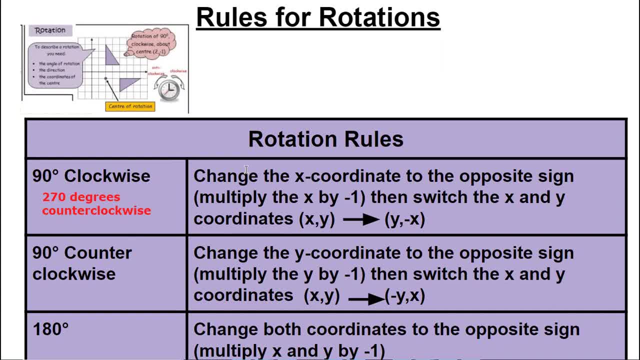 which is the same as multiplying by negative 1.. And then you switch the x and the y coordinates. So here it is. is the example. here x and y would become. switch them y first, then change x to the negative or the opposite value. 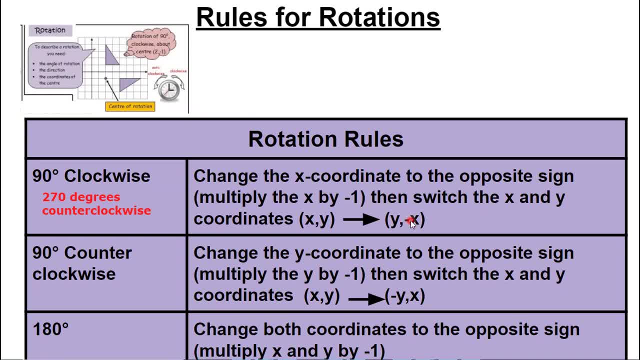 It won't necessarily be negative. If it was negative to start with, it'll be positive. And then we have a 90 degree counterclockwise, And then we have a 90 degree counterclockwise rotation, which is the same as a 270 degrees clockwise rotation. 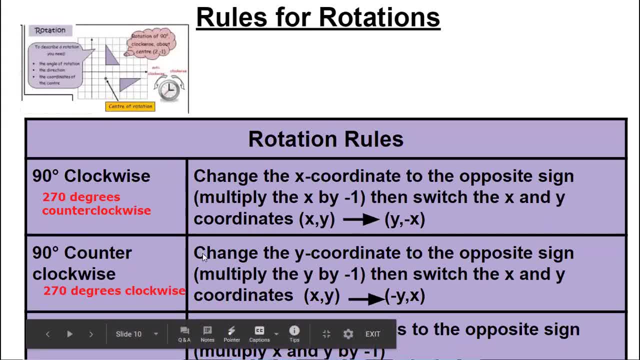 And what you do when you have a counterclockwise 90 degrees? you change the y coordinate. So, instead of the x coordinate, now you're changing the y coordinate to the opposite sign, which is the same as multiplying the y by negative 1.. 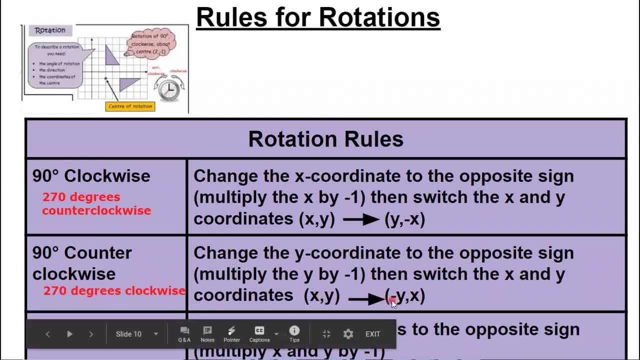 And then you switch x and y, So x and y becomes negative, y comma x. And finally, if you have a 180 degree turn, doesn't matter if it's clockwise or counterclockwise, it ends up in the same spot. 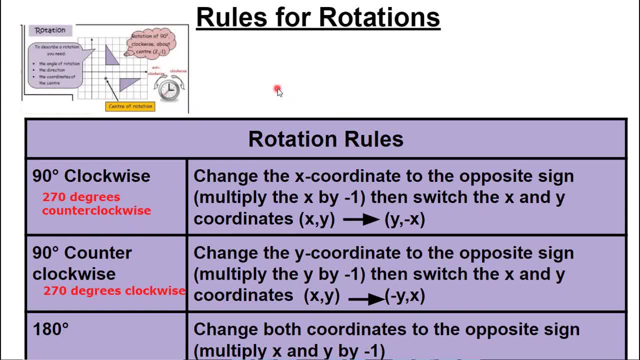 You're gonna change both coordinates to the opposite sign. Don't switch them, just change them to the opposite sign, And I think you can't see it. but you can see it. You can see that down there? No, you can't. 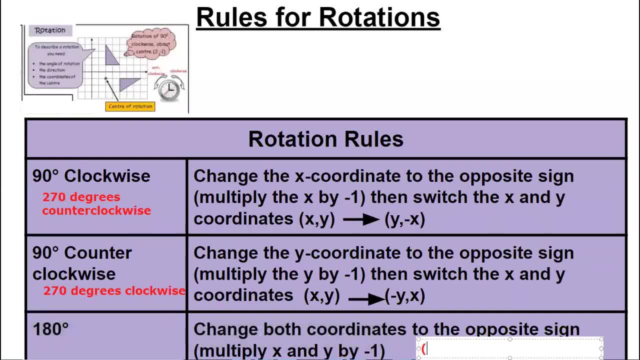 But it said, or it should have said, x comma y will result in negative. x comma negative y. So if they were negative to start with, they'll be positive. If they were positive to start with, they'll be negative. Let's see this in action. 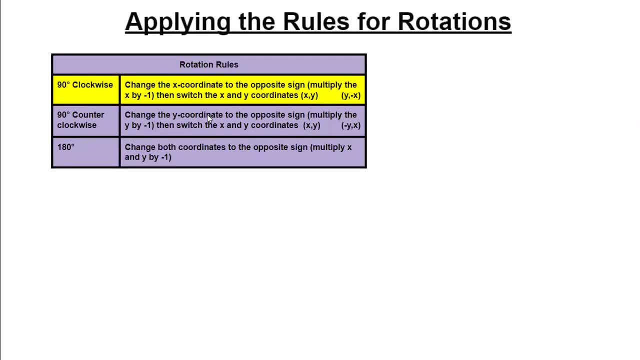 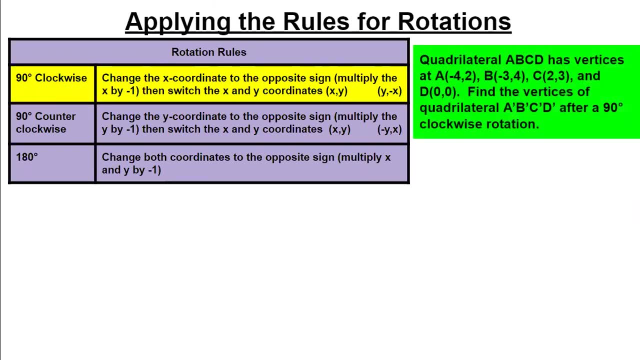 There's our rules Quadrilateral: A, B, C, D has vertices at A negative 4, 2, B negative 3, 4,, C 2, 3, and D 0, 0.. 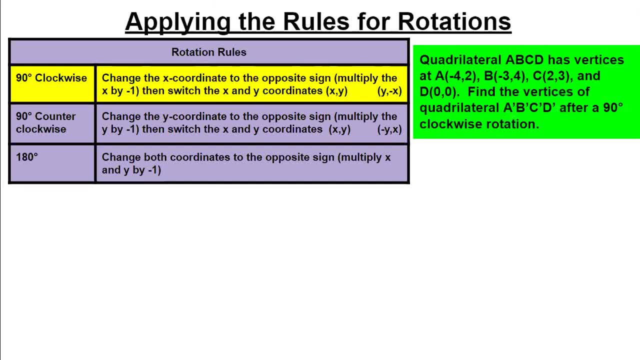 Find the vertices of quadrilateral A, prime, B, prime C, prime D prime after a 90 degrees clockwise rotation. I've highlighted in yellow the rule we'll be using, So let's do that, Okay. So let's plot our points. 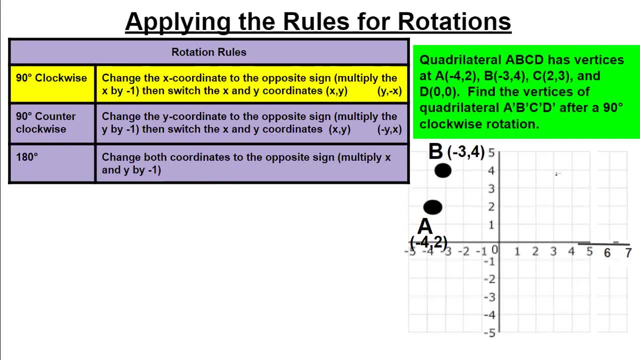 That's A negative 4, 2,, B negative 3, 4,, C 2, 3, and D 0, 0.. Connect the dots. There's our quadrilateral. Okay, Let's bring up our rule. 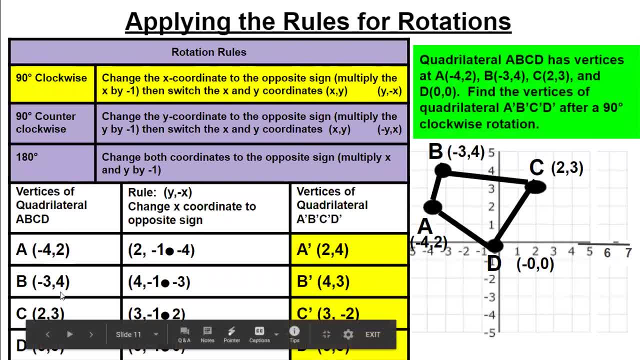 Here's the vertices before the translate or before the rotation. And our rule is going to be up here a 90 degree clockwise. You're going to switch the x and the y, and the x is going to become the negative. Okay. 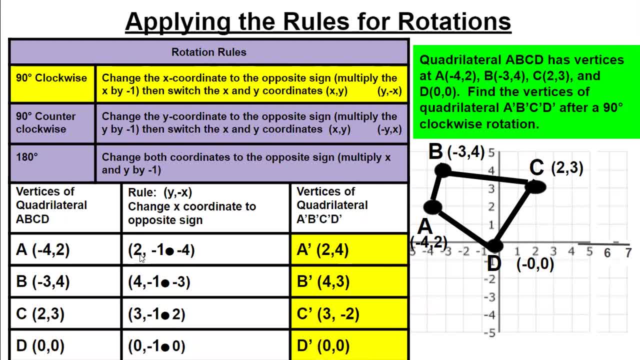 Okay, Or the opposite. I should say: So 2 is going to stay. So here we'd put: the y becomes 2, becomes the x, and then negative 4 becomes the opposite, positive 4.. So we switched the numbers, changed the second value to the opposite sign. 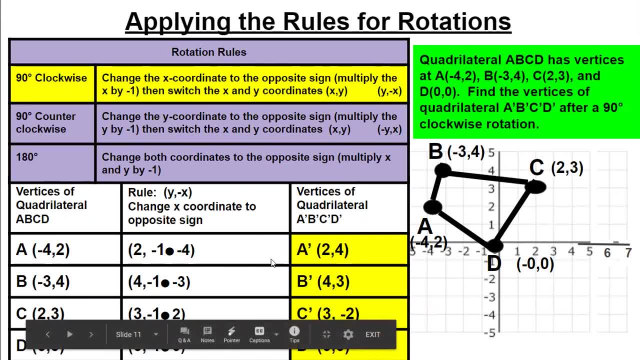 B was negative 3, 4.. Now the 4 is going to be first and the negative 3 is going to change to a positive 3.. For C we had 2, 3.. C prime is going to come with 3, 4.. 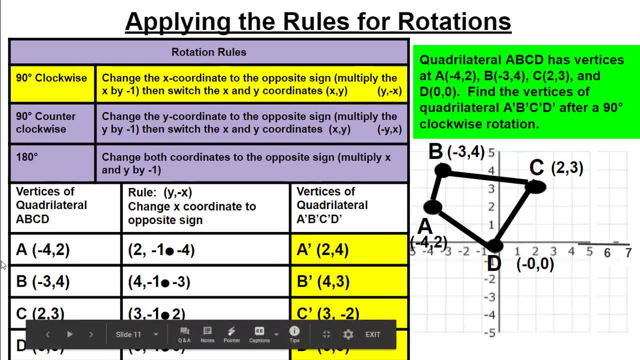 C prime is going to come, with 3 first, and then negative 2, we're changing it to the opposite sign And finally, D is at 0, 0, and notice how 0, 0 doesn't change signs, does it? 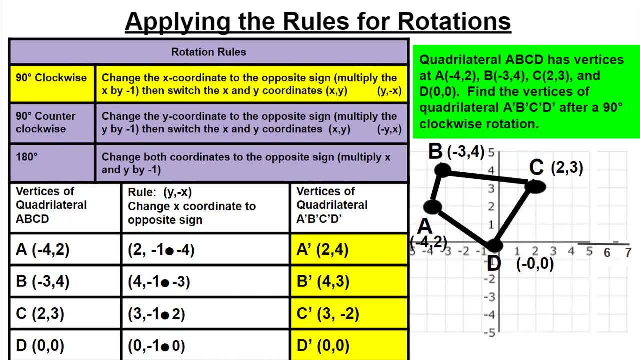 Even when you flip them or switch them around, you get 0, 0 again, So that D point is going to stay in the same spot. Let's plot our vertices. A is at 2,, 4, or A prime, I mean. 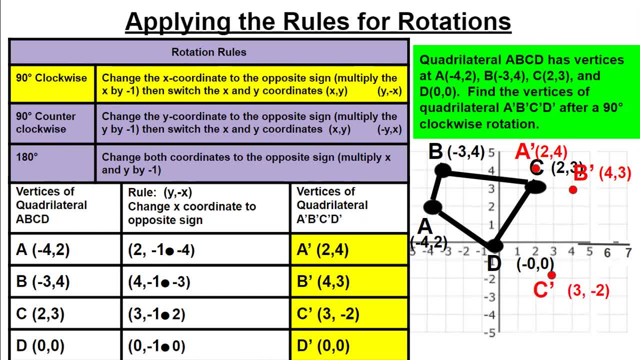 B prime is at 4,, 3.. C prime is at 3, negative 2.. And D prime is at 0, 0.. Connect the dots and there is our rotation, 90 degrees clockwise. All right, your turn again. 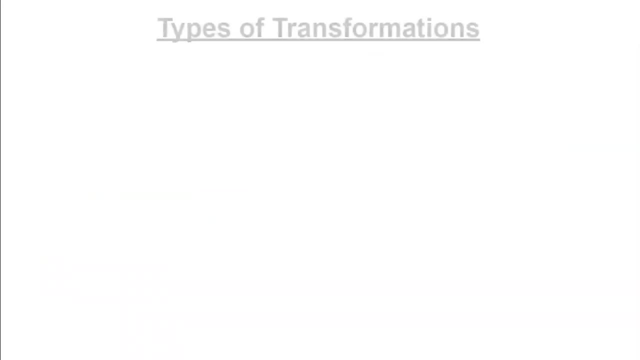 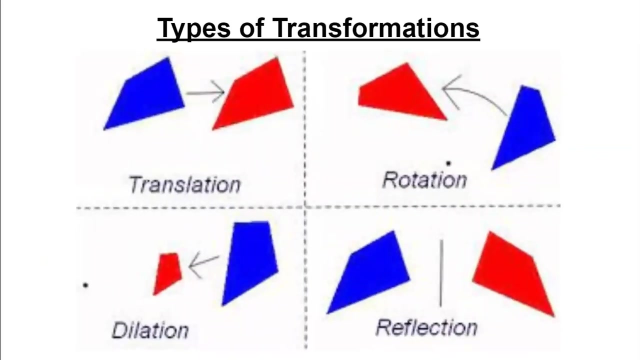 See you back in a minute. Okay, welcome back. Let's take a little bit of a look again. Let's review. A translation is a slide, A rotation is a turn, A reflection is a flip, A dilation is an enlargement or a shrinking. 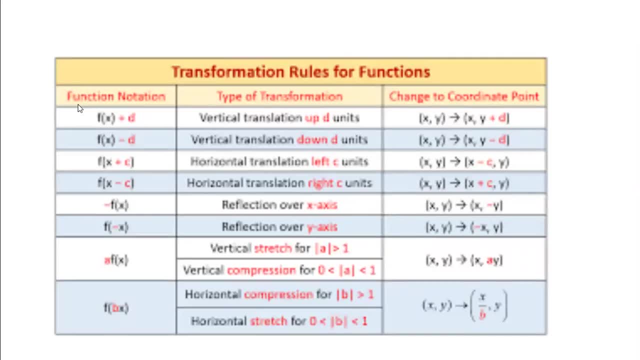 Okay, I just wanted you to be looking at this a little bit. this transformation rules for functions. This is something you're going to deal with more when you get into high school with geometry. I just wanted you to see what this chart looks like. 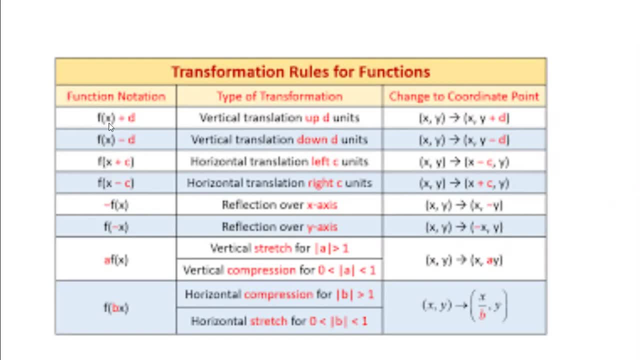 You can kind of make sense of it here: F of X is another word for Y, because that's what a function stands for: plugging in number. So we have a plus D if you translate up D units. We have a minus D if you go down D units. 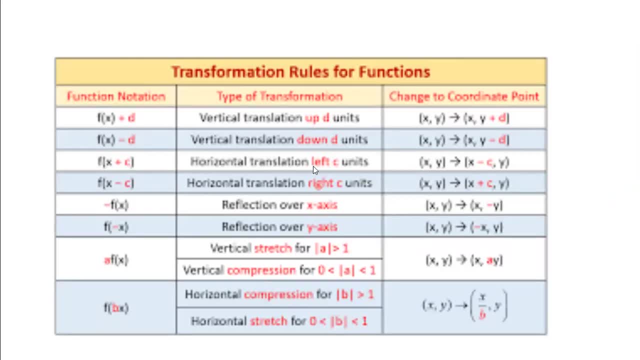 X plus C in the parentheses. if you go a horizontal shift left And X minus C. if you go a horizontal shift, translation right: A reflection: you have an opposite sign here in front. If you have a reflection over the Y axis, the X is changing. 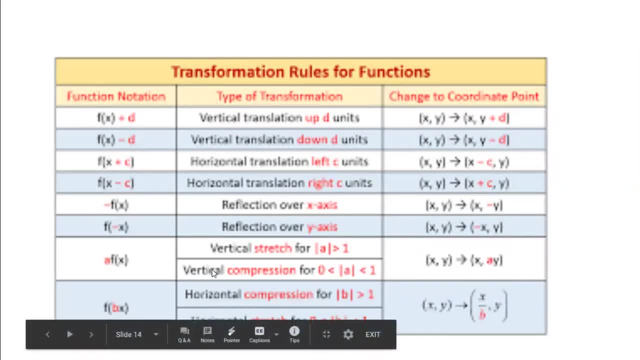 If you have a vertical stretch or compression, that's going to be your dilations. There's different rules for that. You can see you're going to have a coefficient in front of the F of X or a coefficient in front of the X. 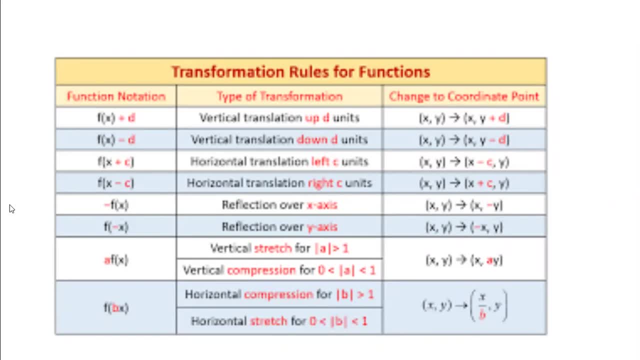 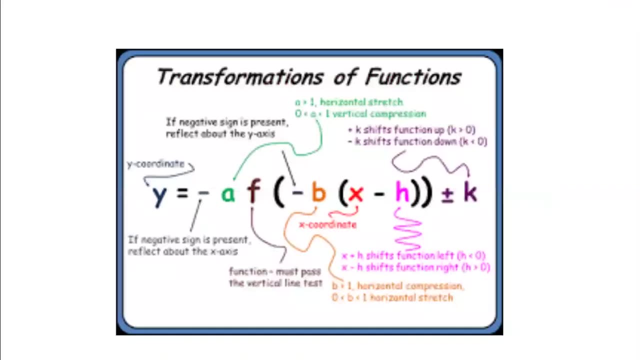 If you want to on your own time. I'm sharing the slides with you. You can take a look at this and delve more into that if you're interested. That was focused on higher order thinking, And this one should have that as well. 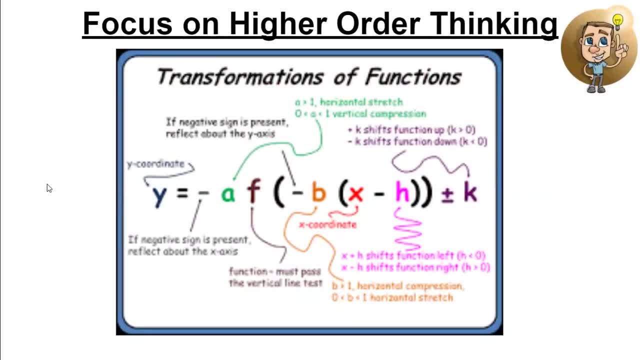 Okay, transformations of functions. I just want you to see that you're going to be also working with equations And every letter stands for some type of transformation. So the Y stands for the Y coordinate. The negative sign represents the How it's reflected about the X axis. 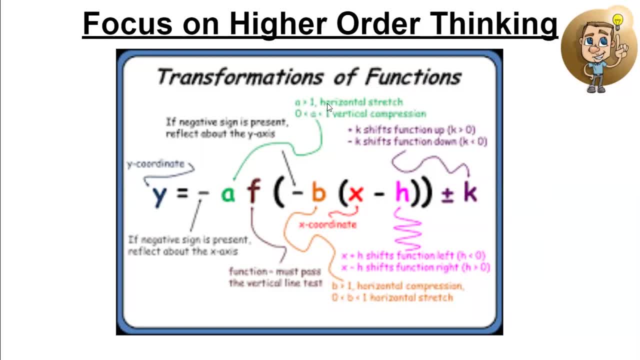 The A represents. if it's greater than one, it's a horizontal stretch. That's a dilation. If it's between zero and less than one, it's a vertical compression or a shrinking. F is a function. Remember: a function must pass the vertical line test. 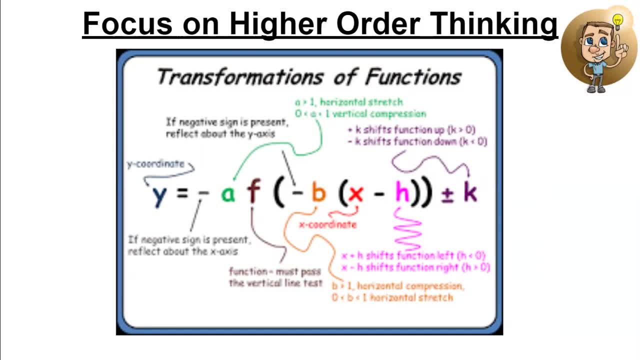 It can only have the same points going vertically but not horizontally. Otherwise it's not a function. This negative sign is present. It reflects about the Y axis. B stands for if it's greater than one, it's a horizontal compression. 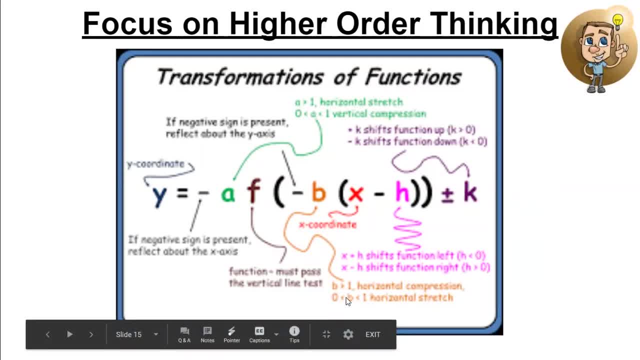 That's a dilation. If it's between zero and one, it's a horizontal stretch. X stands for the X coordinate, The H stands for X plus. H shifts function left For H is less than zero And X minus H shifts the function to the right if H is greater than zero. 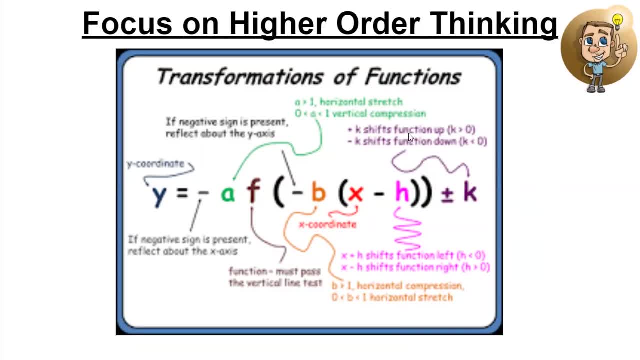 And then you have plus or minus K. If K is positive, If K is positive, then the function goes up. If K is negative, the function goes down. I just wanted you to see that when you get into high school, you're going to be dealing with all kinds of different equations for parabolas and circles. 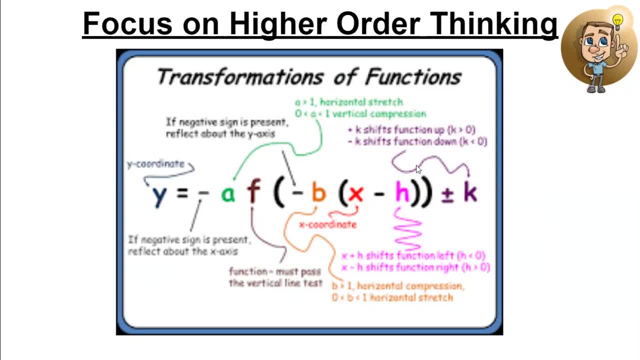 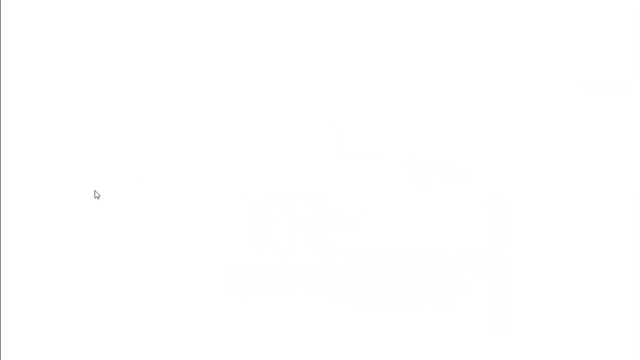 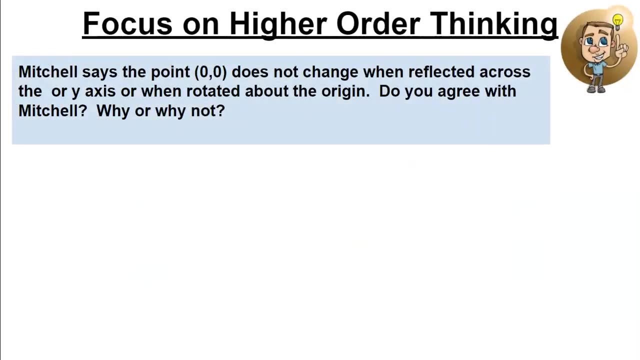 and all these different things. Each one of these letters in an equation represents a type of a transformation from the origin. Okay, let's look a little bit more at higher order thinking. Mitchell says that .00 does not change When reflected across the- it should say X or Y axis- or when rotated about the origin. 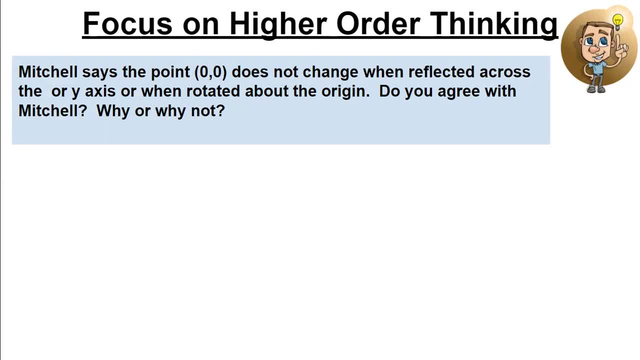 Do you agree with Mitchell? Why or why not? So, when it's reflected, he's saying .00 doesn't change. When it's rotated, he says it also doesn't change. Well, let's take a look, He is correct. 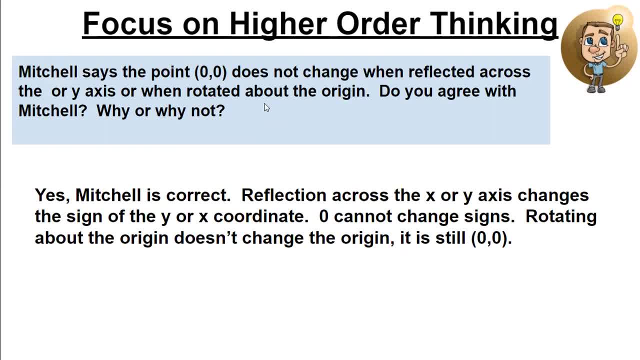 Why? Because a reflection across X or the Y axis changes the sign of the Y or the X coordinate. Zero cannot change signs, So it would still be .00.. Rotating about the origin also doesn't change the origin. It is still .00.. 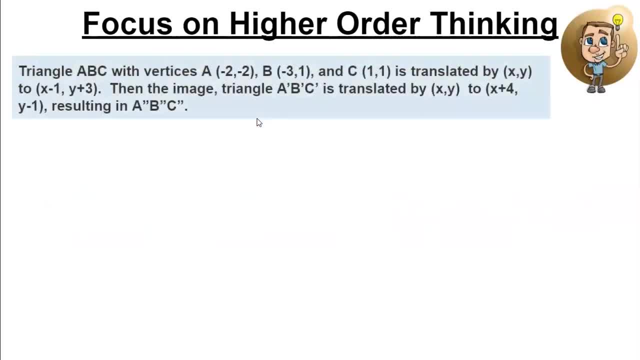 Zero Triangle ABC has vertices A negative 2, negative 2,, B negative 3, 1, and C 1, 1.. It is translated by XY to the point of X minus 1,, Y plus 1, and Y minus 1.. 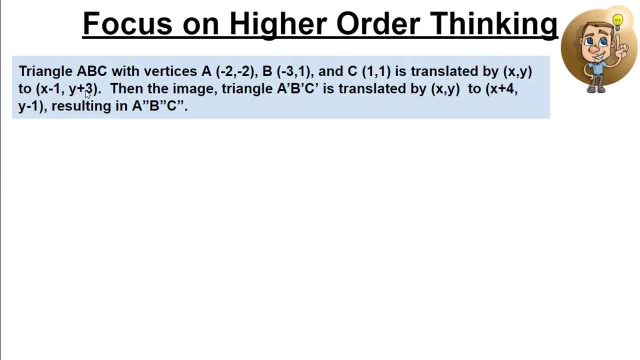 Then the image triangle A prime, B prime, C prime is translated by XY to the X plus 4, Y minus 1, resulting in A double prime, B, double prime, C, double prime Sounds like a lot. It's not as bad as it looks. 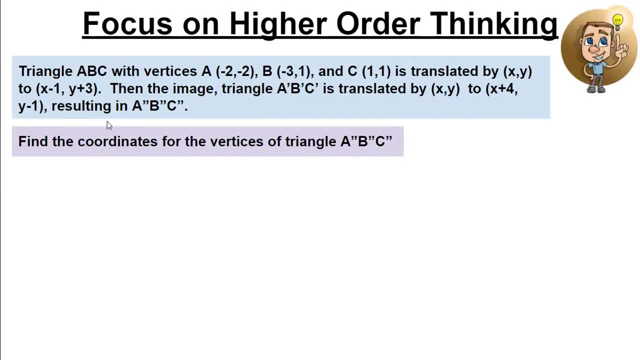 Find the coordinates for the vertices of triangle A double prime, B, double prime, C, double prime. To get to that we have to do two steps. Step one: We have to find A prime, B prime, C prime. So we're going to subtract 1 from A. 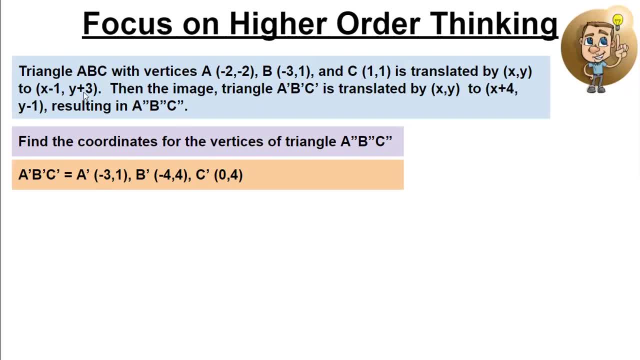 So negative 2 minus 1 will give us negative 3.. We're going to add 3 to the Y coordinate, which is negative 2. Adding 3 gives us 1. B prime. we're going to take 1 away from negative 3.. 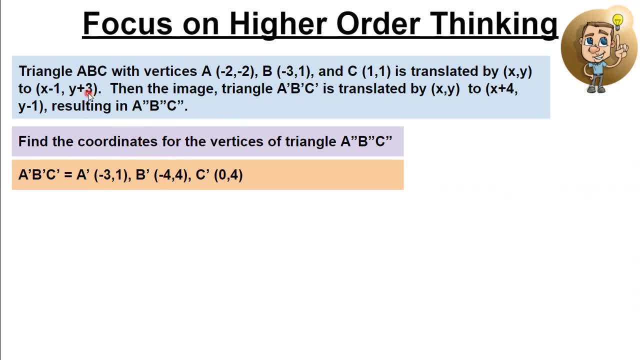 That makes negative 4.. We're going to add 3 to the Y value, which gives us 4.. C prime: We are going to take 1 away from the value of X. 1 minus 1 is 0.. We're going to add 3 to the value of Y. 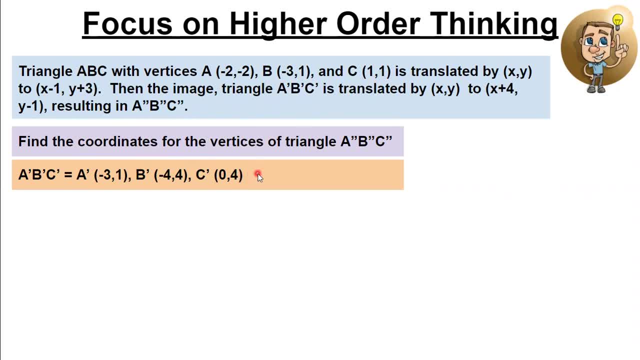 1 plus 3 is 4.. That's A, B and C prime. right Now we have to do it again for a translation of X plus 4 and Y minus 1.. So A is going to add 4 to what we had here. 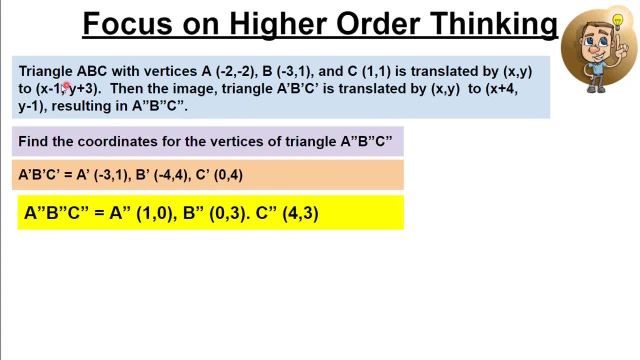 So negative 3 plus 4 becomes 1.. It's going to subtract 1 from the Y value. 1 minus 1 becomes 0.. It's going to add 4 to negative 4.. That becomes 0. It's going to subtract 1 from 4.. 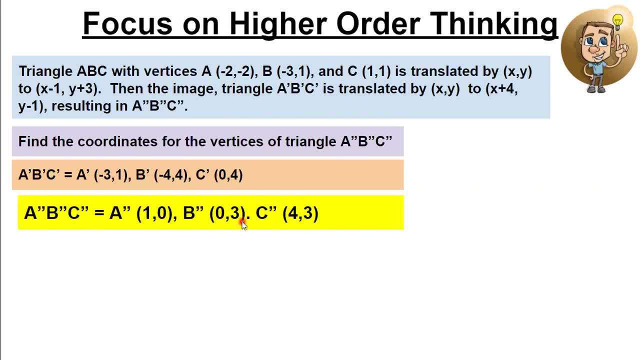 4 minus 1 is 3.. And then C prime was 0. We're going to add 4 to that, And the Y value was 4. And we're going to subtract 1.. So 4, 3.. 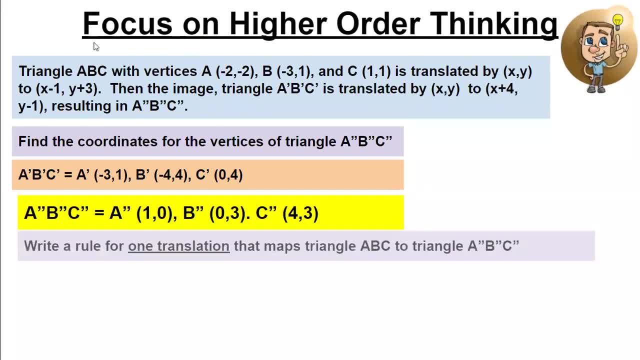 It wasn't as bad as it looked. Write a rule for one translation that maps triangle ABC to triangle A prime B prime C prime. To map the triangle means to put it in the same spot. So after two translations up here, what one translation can you make to get the first triangle ABC to be? 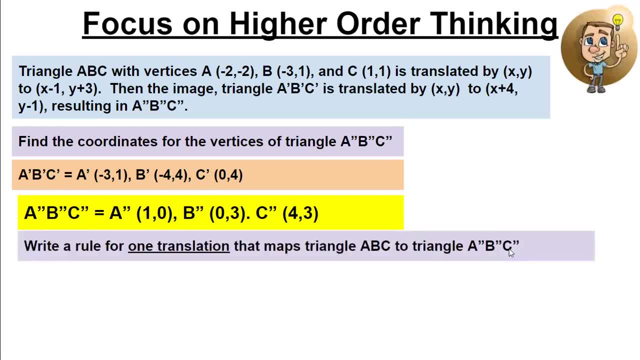 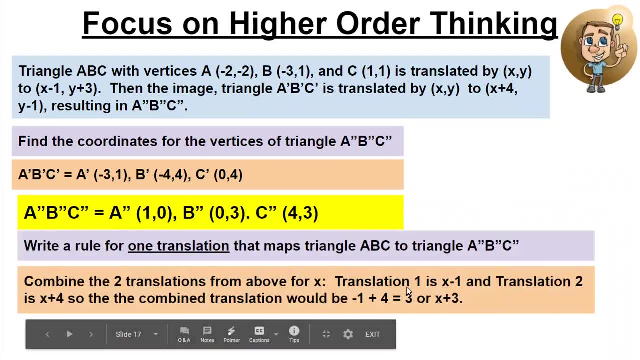 A prime, B prime, C, prime in one step. Well, you have to combine the two translations from above for X. What was the first translation? One was X minus 1.. Let me get my spotlight here: X minus 1.. 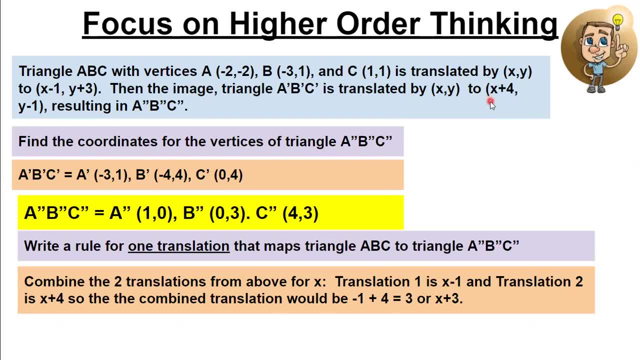 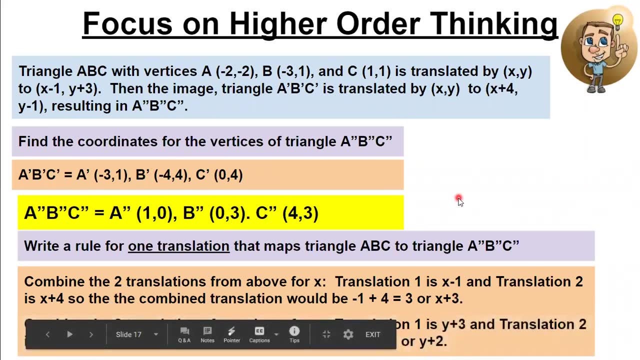 The second translation was X plus 4.. So then you're going to add them together: Minus 1 plus 4 is equal to 3.. So a one-step translation would be X plus 3.. And then Move my black bar there. 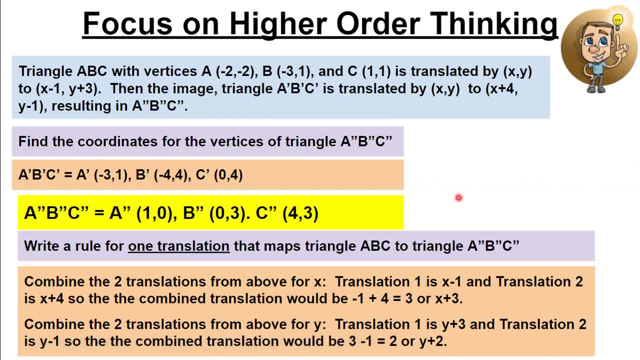 You're going to combine the second translation for the two translations for Y. Translation 1 was Y plus 3.. Translation 2 was Y minus 1.. So you're going to add 3 plus negative 1 or 3 minus 1..